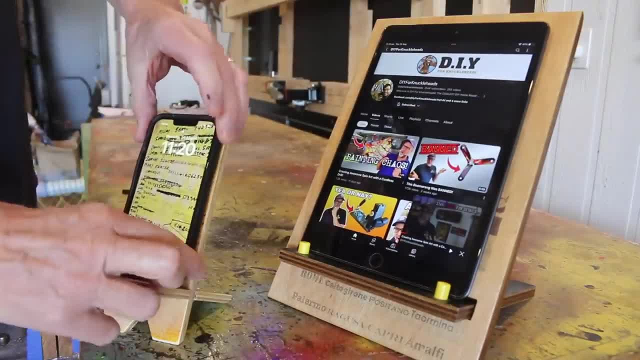 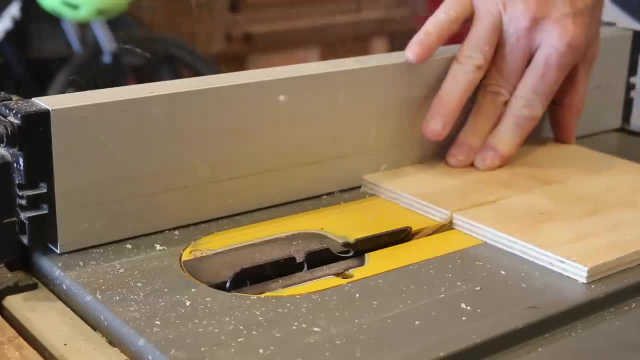 which makes phone and tablet stands like the ones you see here a very popular thing to sell Now. the cost of materials to make one of these is very little, which is great for your profits, And the time to make one is very quick. 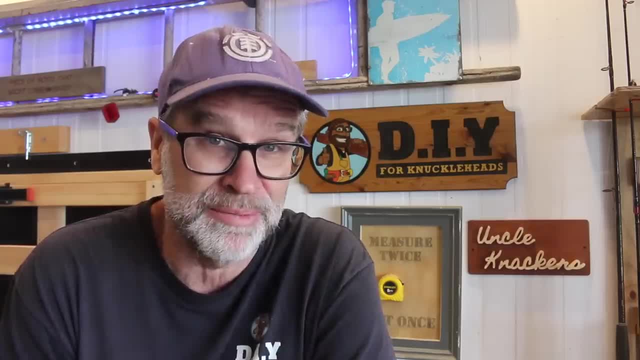 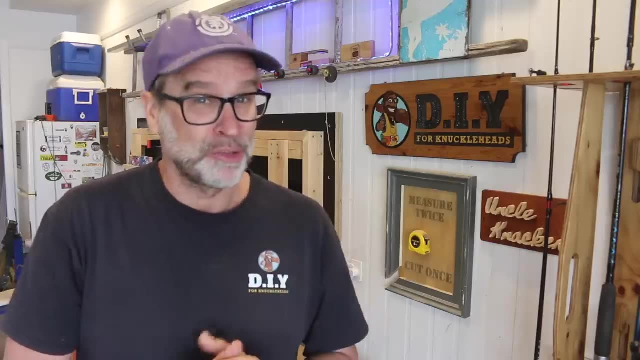 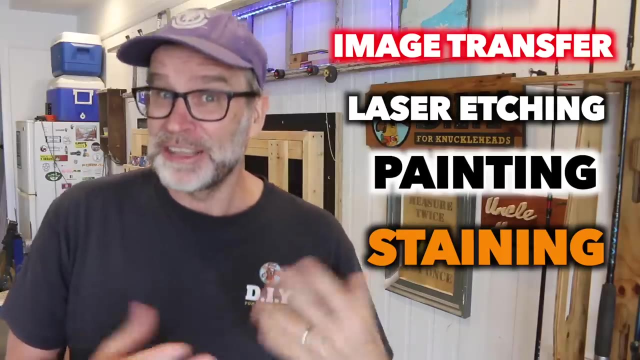 especially if you use a template to mark out the pieces. Now, in regard to customization, to make yours stand out from the crowd, the sky's the limit, with many options available, such as image transfer, laser etching, painting, staining, et cetera, et cetera. 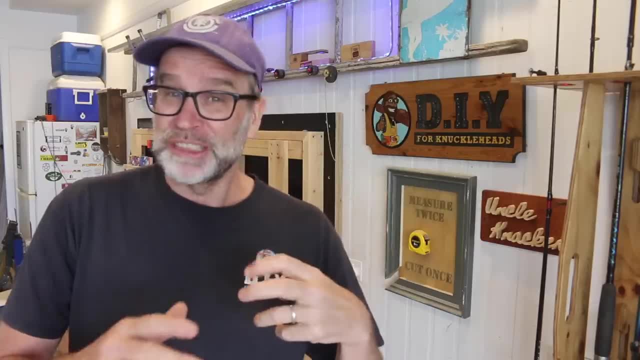 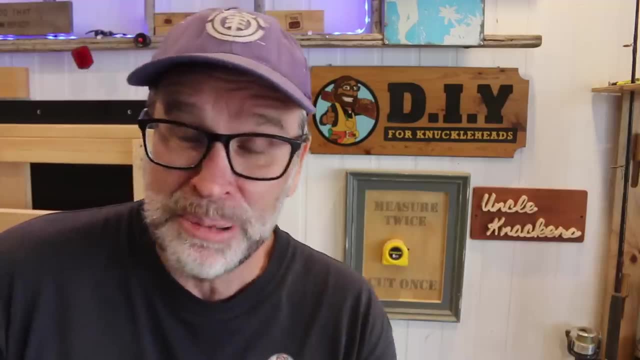 But just remember, the more complicated the finish, the longer it's going to take, which means the less profit you're going to make. And don't be afraid to use that old, classic marketing ploy from McDonald's regarding the do you want fries? with that upsell technique. 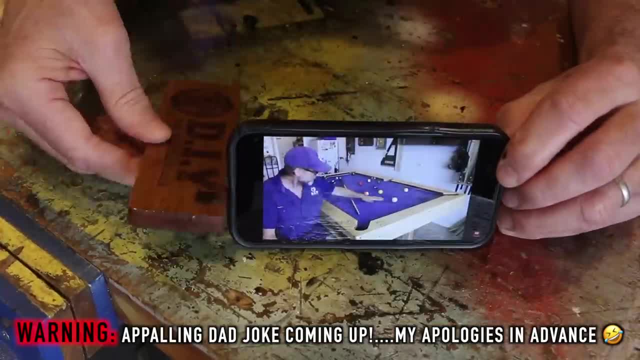 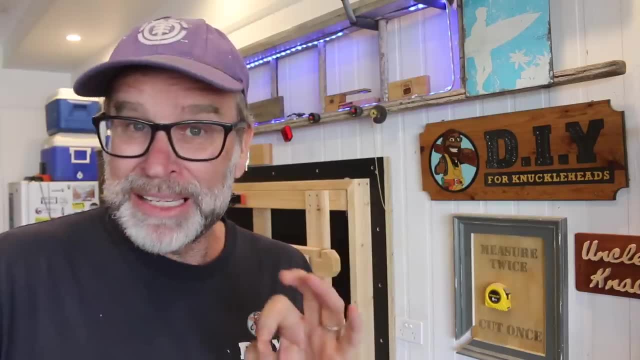 which, in this case, could come in the form of a smaller item like one of these little phones. phone stands as an extra purchase. Hey, since we're talking about phones, how's this? A couple of days ago, I called my wife. 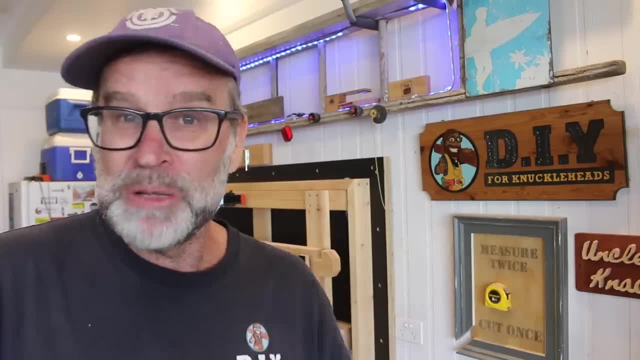 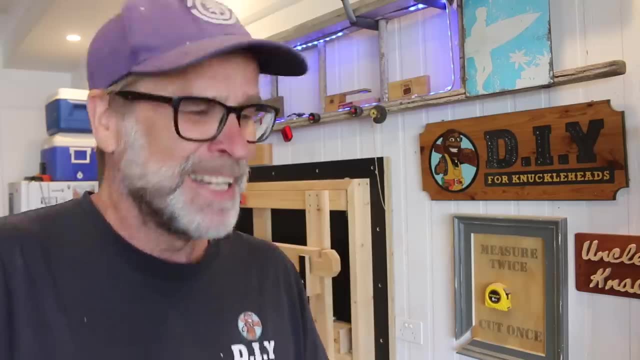 and she was driving home from work And I said, hey, hang on a sec. I've just been watching the news and apparently there's a maniac driving down the wrong side of the road, not far from where you are, And she says one. 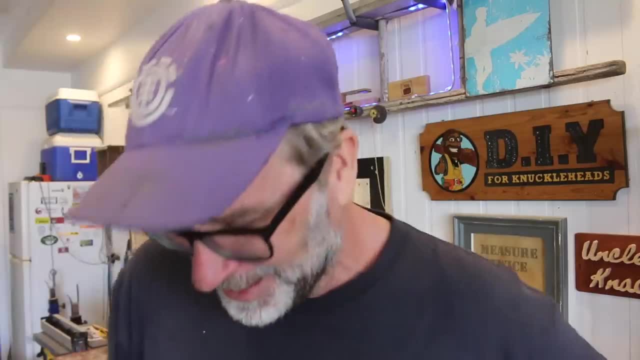 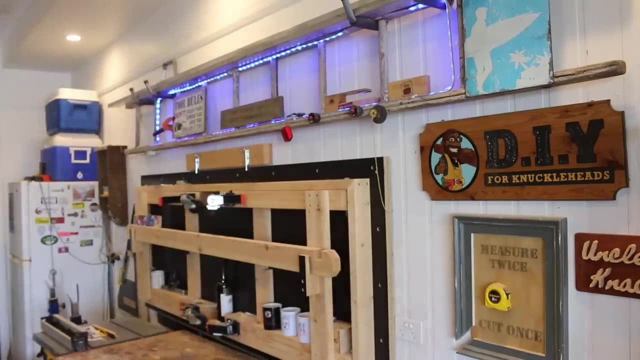 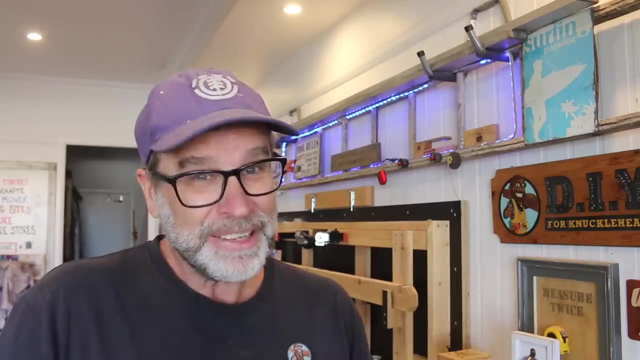 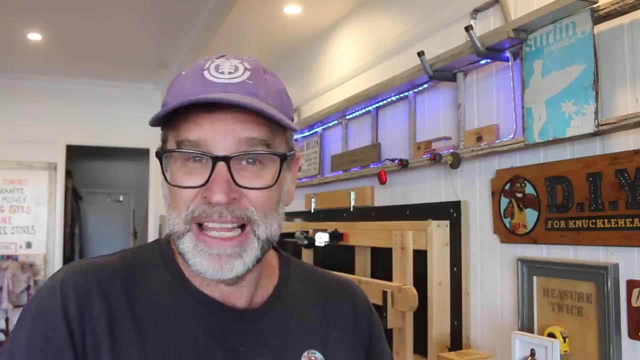 There's hundreds, It's always one. Oh dear, oh dear. Now look, let's face it. Lots of people drink beer And, as a consequence, any beer related type product tends to be a good seller, such as something like this: wall mounted bottle opener. 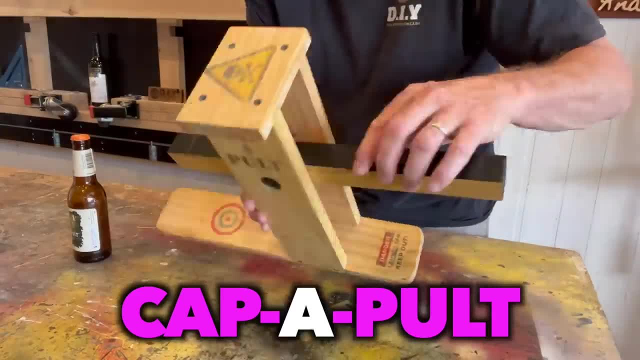 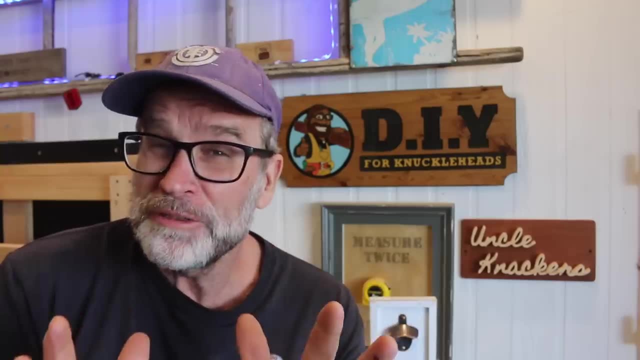 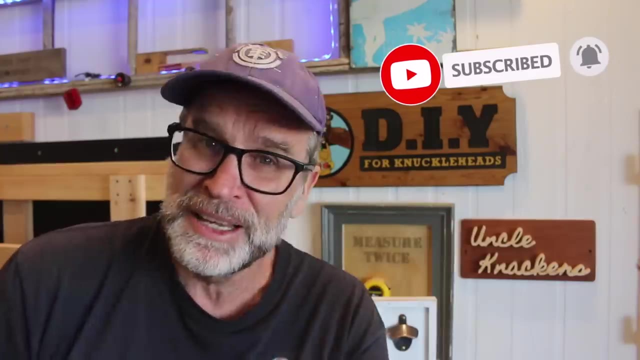 made from recycled pellet wood, or the awesome Cappapult which can launch those pesky bottle caps with ease into the outer stratosphere. Both of these are really fun products and a great gift ideas for things like Father's Day, birthdays, Christmas, et cetera, et cetera. 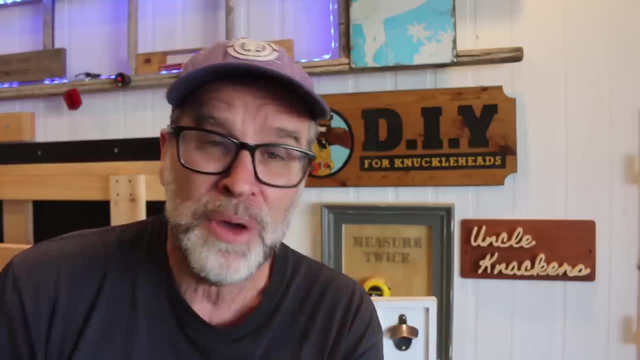 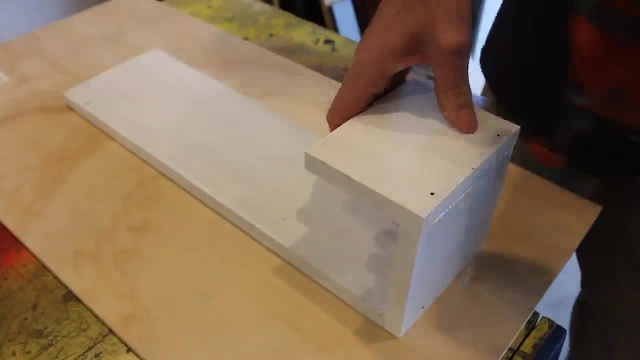 And they look great mounted next to a barbecue or in a man cave. Now, both of these products are cheap and quick to make, but what I really like is the fact that they are very demonstratable, which is great if you're trying to attract people. 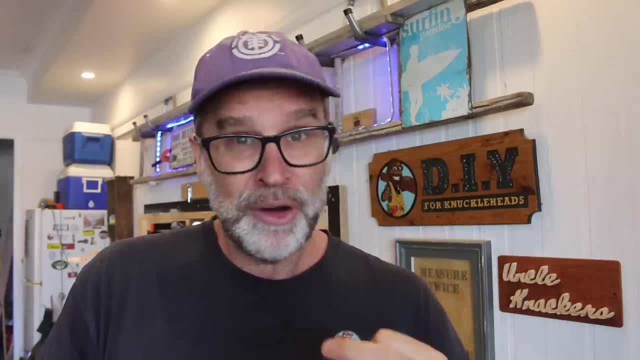 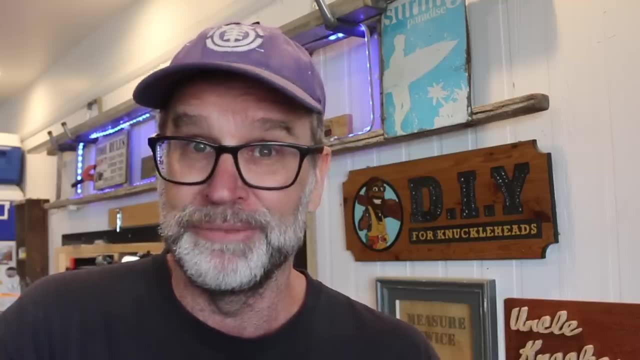 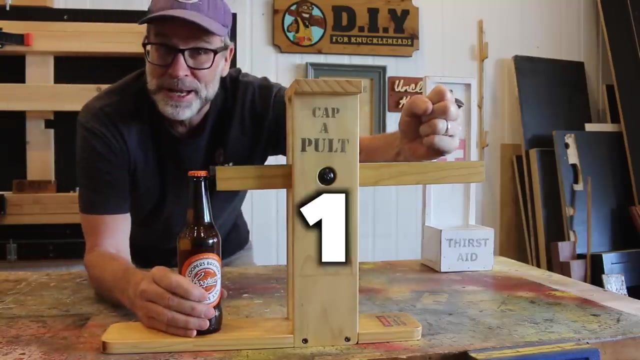 to your market stall, or if you want your product, via a video demonstration, to stand out from the competition when selling online. for example, Stand back folks. This could go anywhere. Righto, here we go. One, two, three. 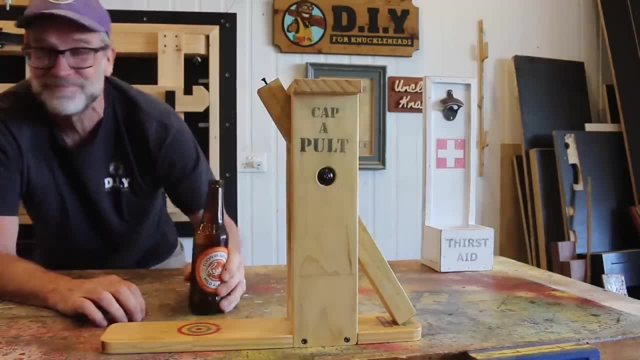 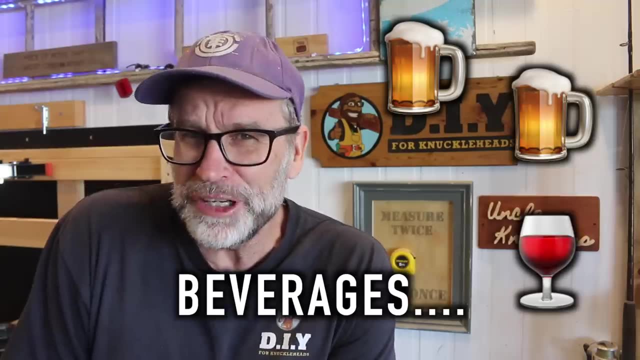 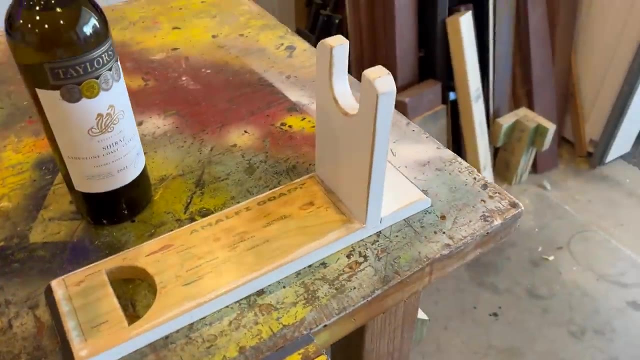 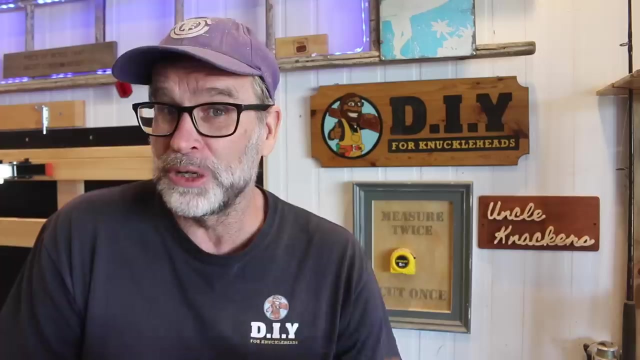 That is awesome. Cheers. Now sticking with beverages. I can see a theme building up here. Wine bottle stands like this one are great sellers and have a good profit margin, as it's basically just two small boards screwed together. And the really good thing about this product: 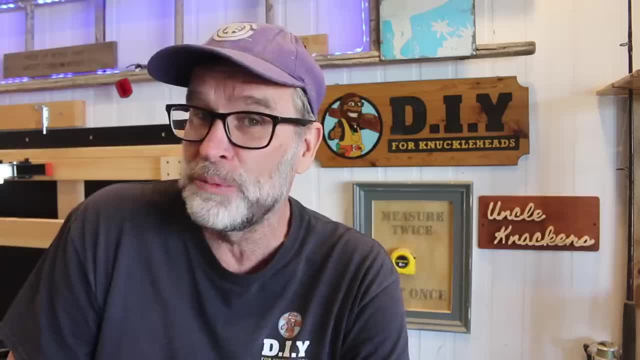 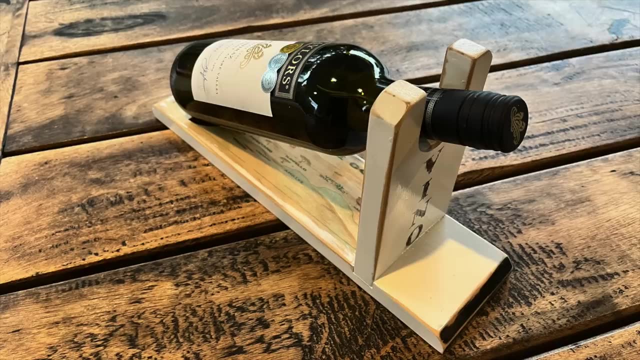 is that you can batch out four of these out of the one 2.4 metre or eight foot stick. You can also make yours stand out from the crowd by either painting, staining, etching, et cetera, Et cetera, et cetera. 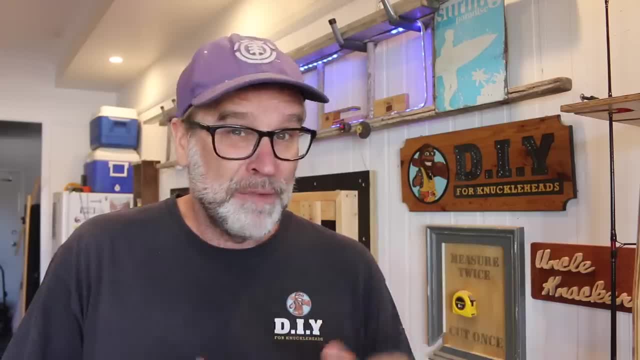 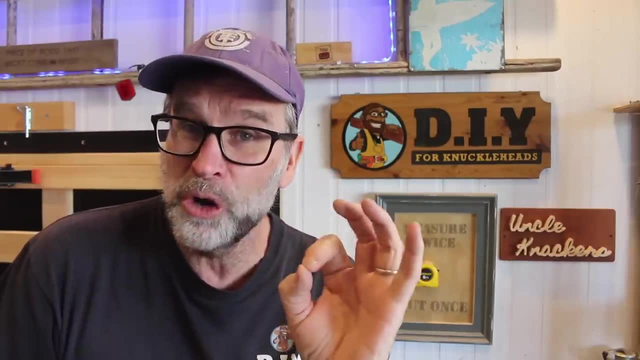 And they also look great just the way they are, if you can find yourself a nice rustic piece of wood. Now, two quick things worth noting. Number one is that you can make these wine bottle stands using basic tools which most woodworkers have in their workshop. 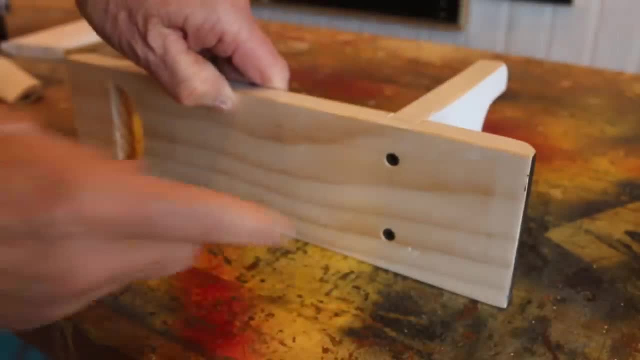 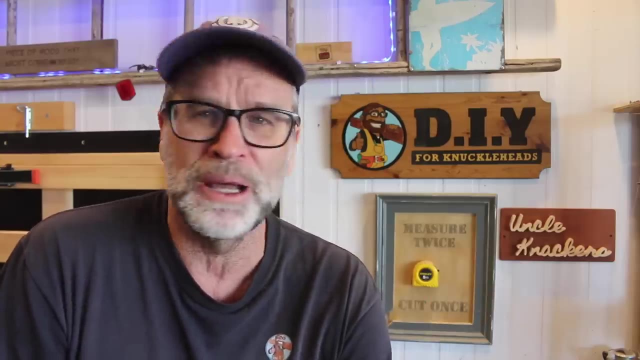 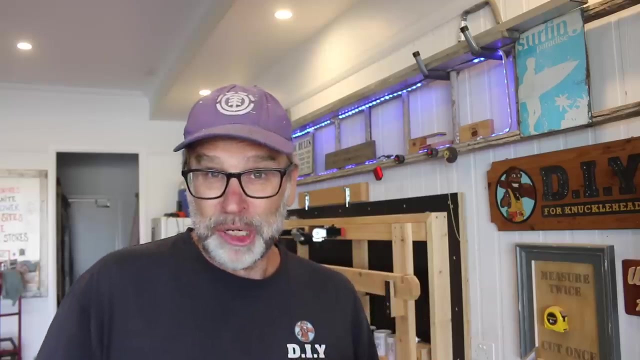 And number two is that you can also flat pack the product by simply unscrewing the two pieces, which makes shipping cheaper. That's hard to say: Shipping cheaper, shipping cheaper. And for the fifth product, let's mix things right up with a really fun project. 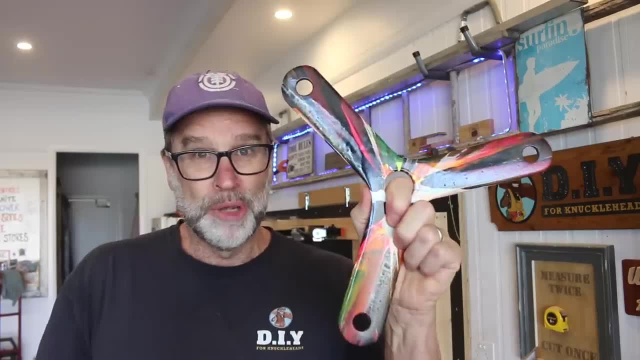 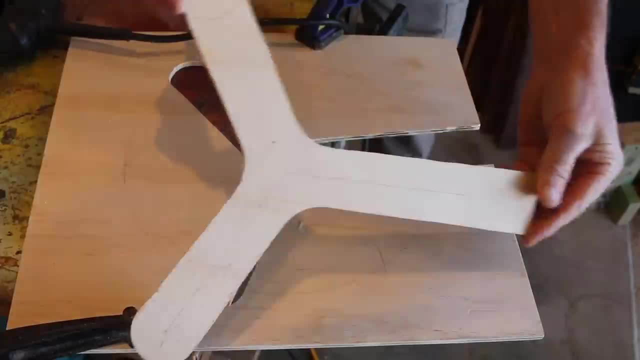 because guess what? Boomerangs are back, baby. And the good news is that they are very easy to make once you know a few of the tricks and cost very little to produce. And what I love is that they grab people's attention. 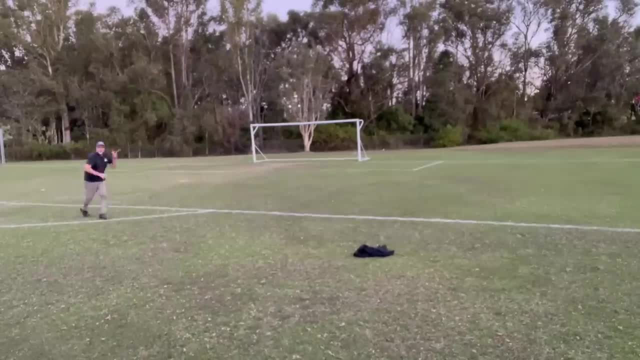 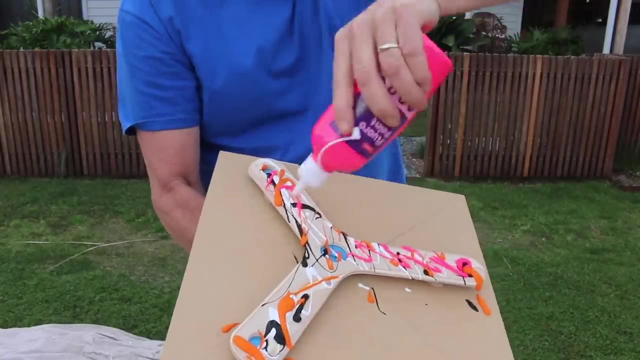 They appeal to all ages And they're great fun to fly. Now the key is to make yours unique so it stands out from all the other boomerangs out there. For example, in the video I used the technique of spin art to finish mine. 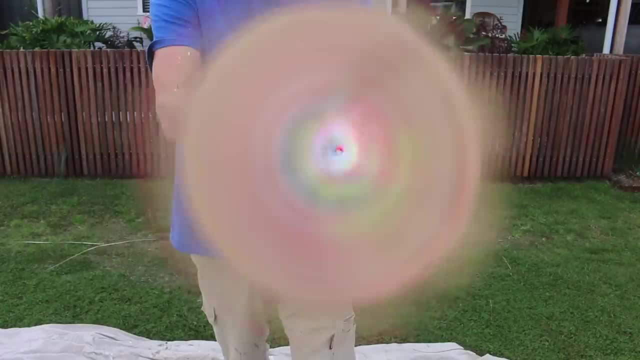 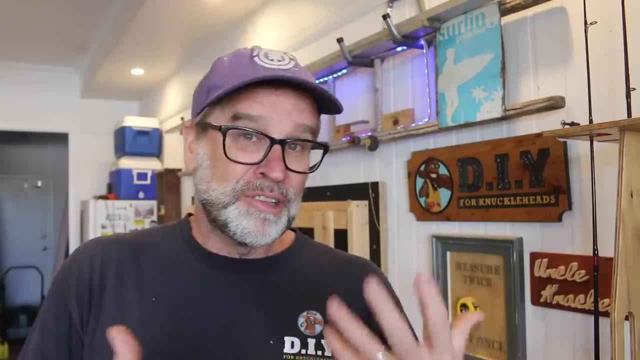 making every boomerang different, which means that you can bump up your price a little, as you can sell it as a one-off product, emphasising the fact that it's the only one of its kind And because it's light and thin. 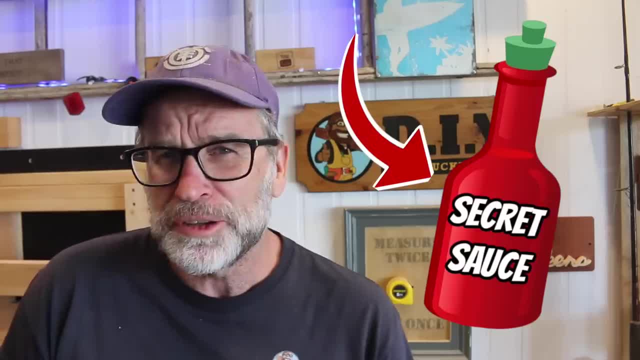 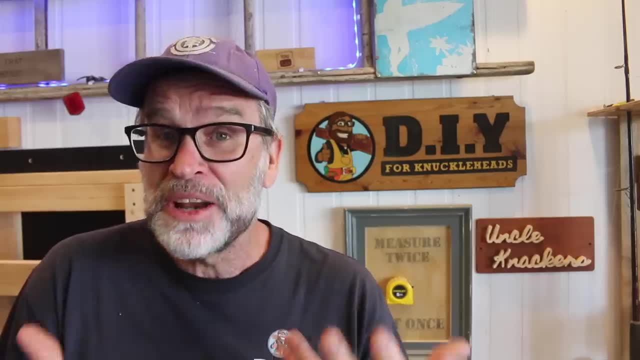 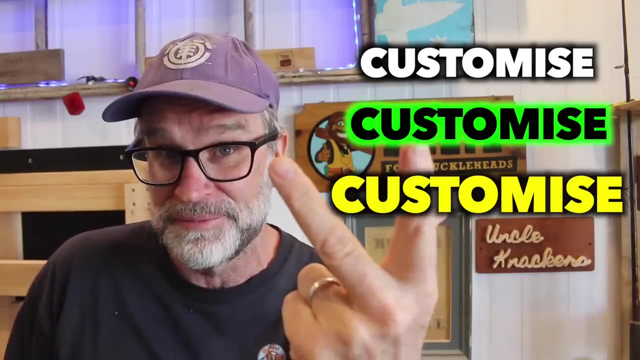 the shipping costs are very low. So what's this secret sauce to making more sake And what's the secret to making more sales that I alluded to earlier in the video? Well, listen up, because here it is, in three simple words: Customise, customise, customise. 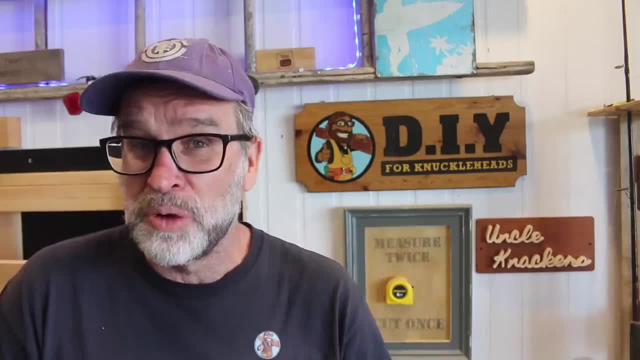 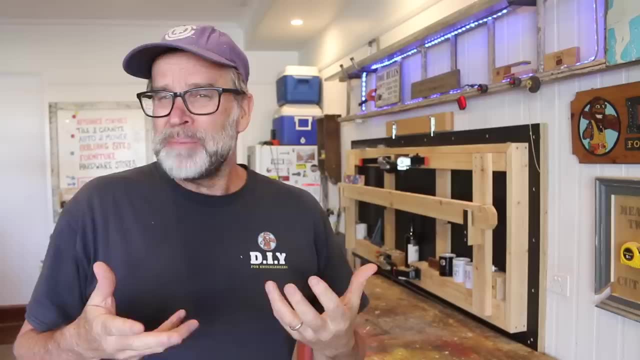 I know it sounds obvious, but you need to cater to your customer's wants, which really is just business basics 101.. Now, using the wine bottle, stand as an example. maybe you could offer five different stain or paint options. You could engrave somebody's name on it. 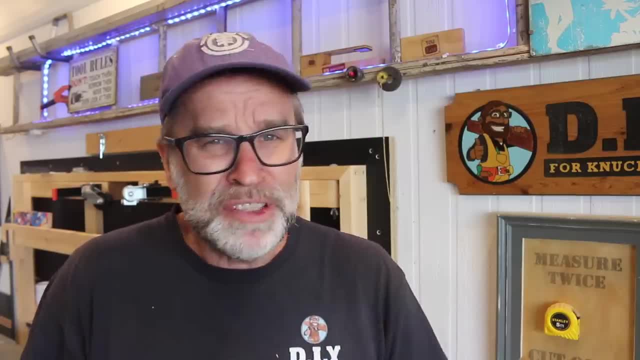 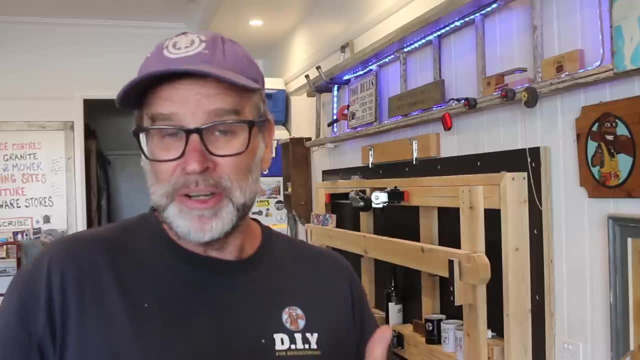 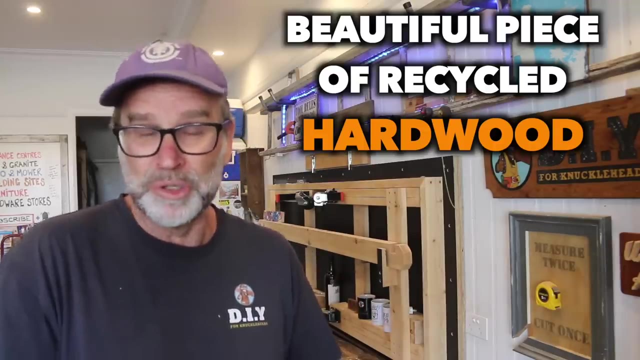 Because personalising stuff sells. People love seeing their names on things. It makes it personal and more sellable. Or maybe offer the product in various materials. For example, along with the one that you made from pine, offer one made from a beautiful piece of recycled hardwood. 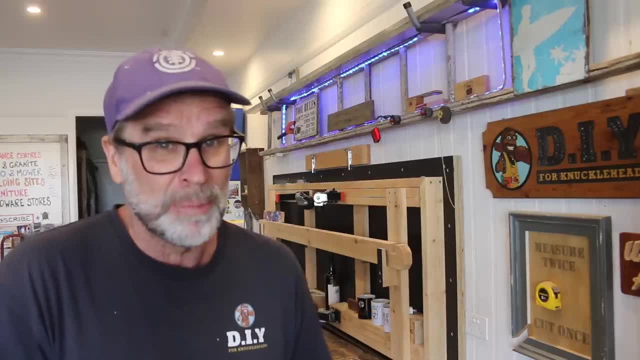 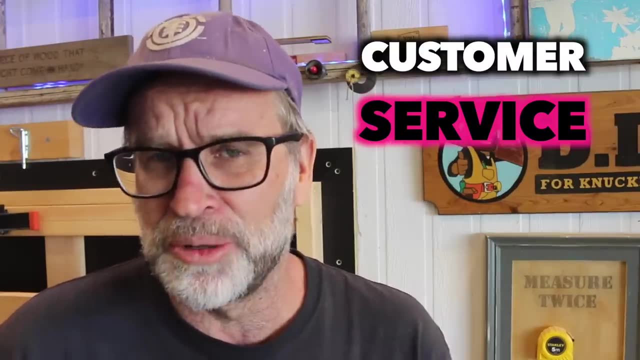 which you can charge a little more for and can also help to drive up sales. And again, business basics 101, when it comes to customer service, which is very important, by the way, and that is just. remember that it takes a lot of time and effort. 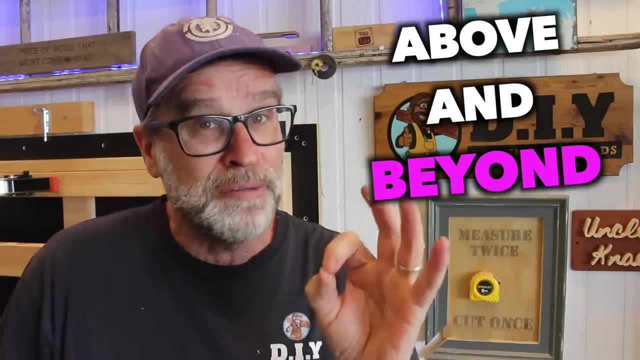 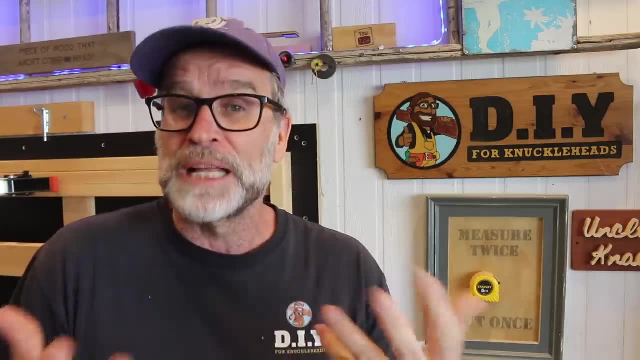 just to get one customer. So once you get one, go above and beyond what people expect and you'll find yourself with a loyal, constant stream of return customers, which relates to more money in the bank And, let's face it, that's why you set up the side hustle in the first place. 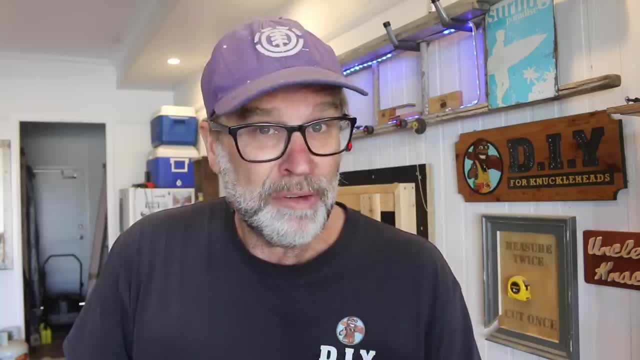 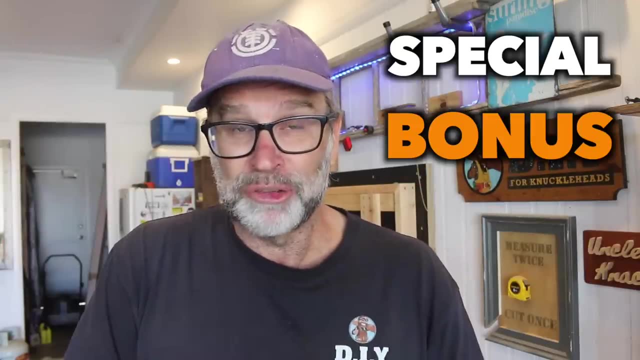 Now, if any of those project ideas take your fancy, do yourself a favour and check out the description box down below where you can access all those plans, And I'll even throw a link in the description box below and throw in a special bonus for those of you. 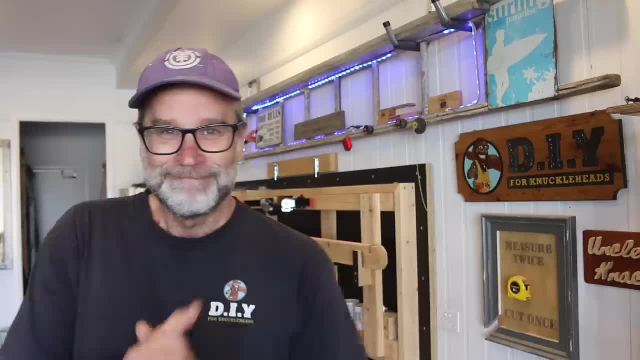 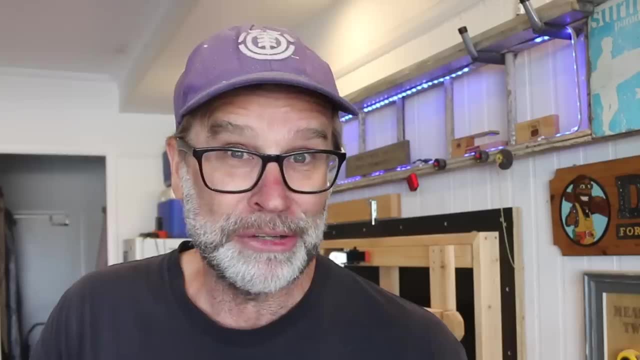 who want to take their woodworking side hustle to the next level. Alrighty, I wish you all the best with your woodworking endeavors, And after all that, I think I need a cup of tea. So until next time, be good, be safe. and I'm out of here, Cheers.